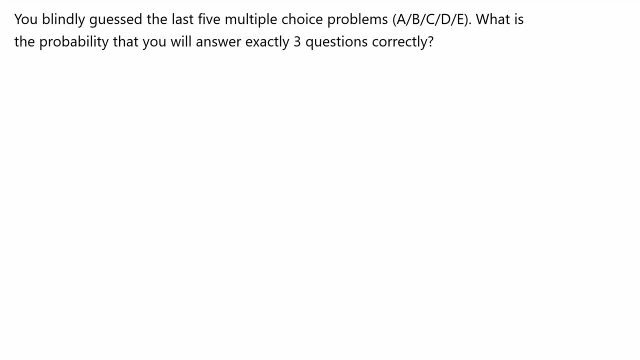 Hello guys. so today I'm responding to a comment in one of my probability videos. You blindly guessed the last five multiple choice problems. So these are multiple choice problems where you have five choices- A, B, C, D, E- And what is the probability that you answer exactly three questions correctly? 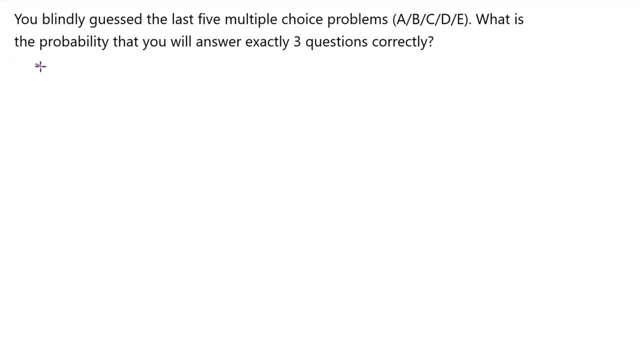 First of all just explain the question. So, basically, you're going to answer five questions- one, two, three, four, five, five- and you are going to kind of put down your guesses maybe, maybe something like this: 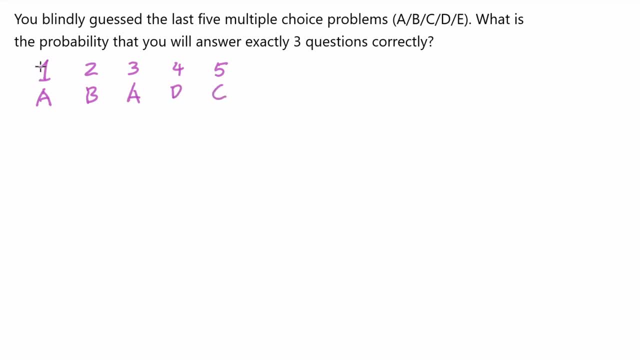 I'm just making it up So you might get some question correct and maybe some incorrect, And we are interested in the problem. The probability that you get three of them correct, The probability of getting one question correct: if you guess randomly, that would be one over. 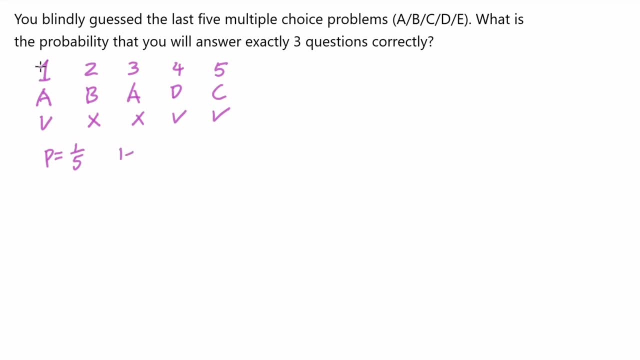 five, And the probability of getting that wrong would be just one minus that. So let's apply the binomial distribution formula directly. So I'm going to write down the formula: P of K, P of K Equal to N, choose K times P of K. one minus P to the N minus K. 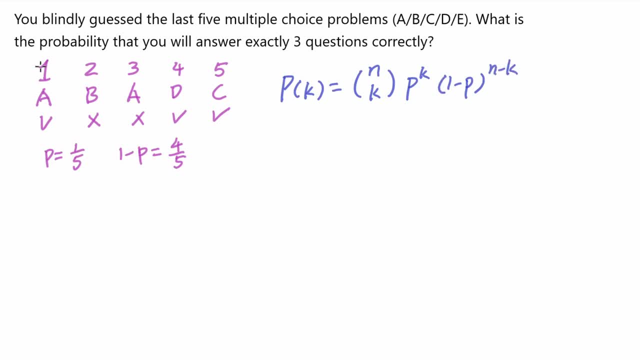 Basically, N is five in this example and K would be equal to three. So in this particular example, P of K equal to three would be three. Okay, So that would be five, two, three times one over five, cube and four over five. 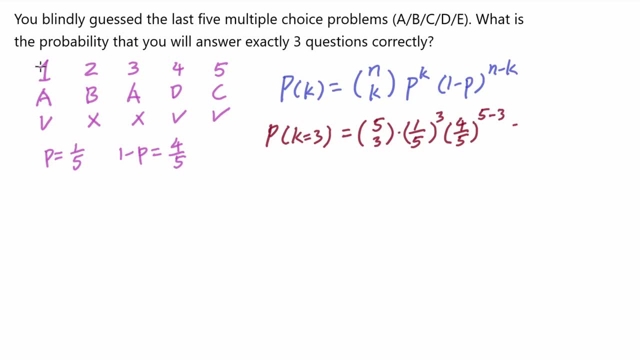 So five minus three, so that would be square, And which I plug it into the calculator, you should get something about 5%. Why does it work this way? Okay, So let's go through the logic, right? So if you look at this. so how many ways are there to answer five questions and answer?